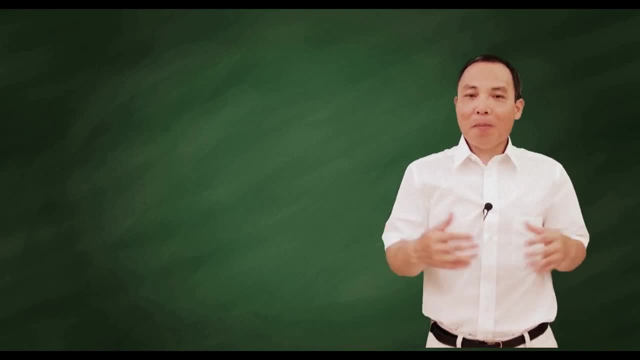 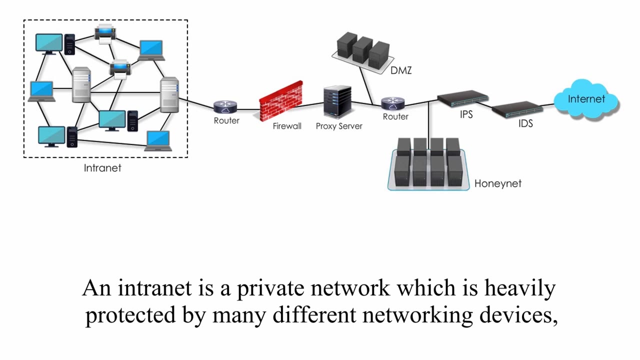 Hello, and this is Sony. Welcome back. An intranet is a private network which is heavily protected by many different networking devices, such as router, firewall, proxy server, DMZ, HoneyNet, IPS and IDS. This diagram is an overly simplified version of the reality. 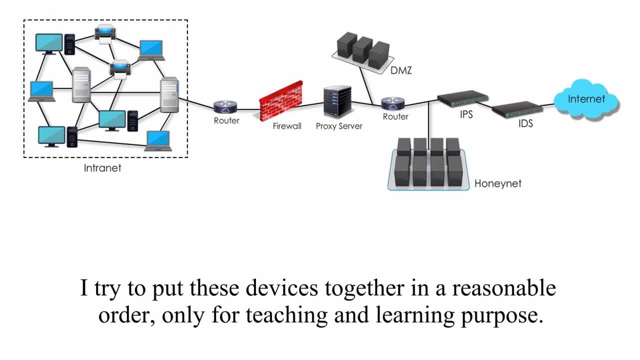 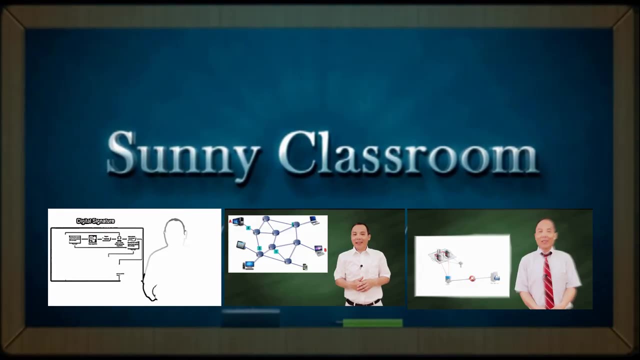 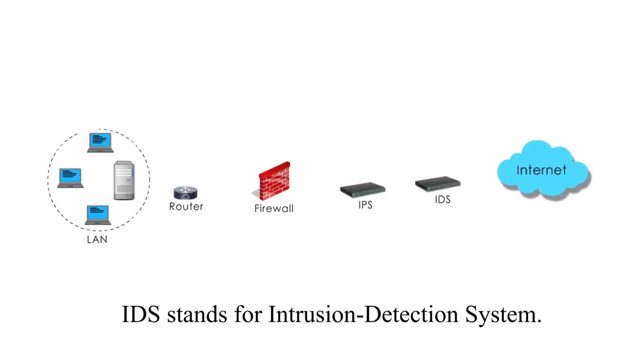 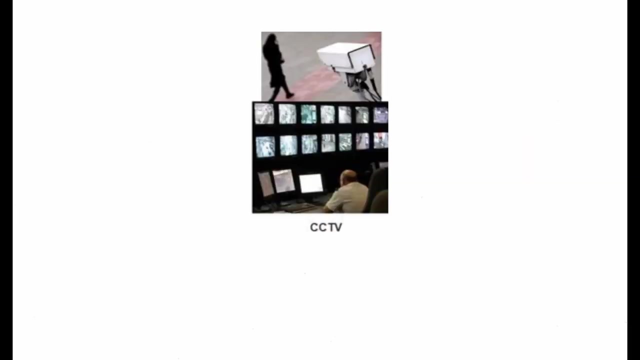 I tried to put these devices together In a reasonable order only for teaching and learning purpose. Today, my topic is IDS and IPS. IDS stands for Intrusion Detection System. The system is often deployed on the network close to the parameter. It is very much like IP. 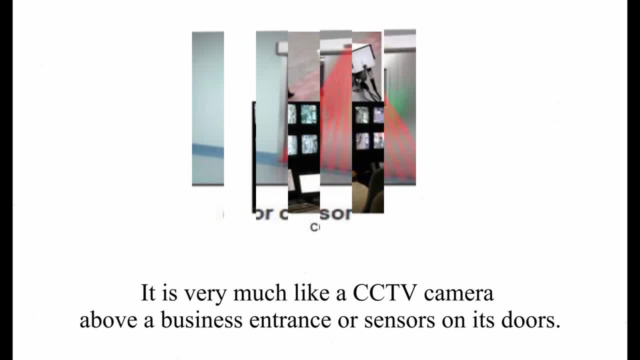 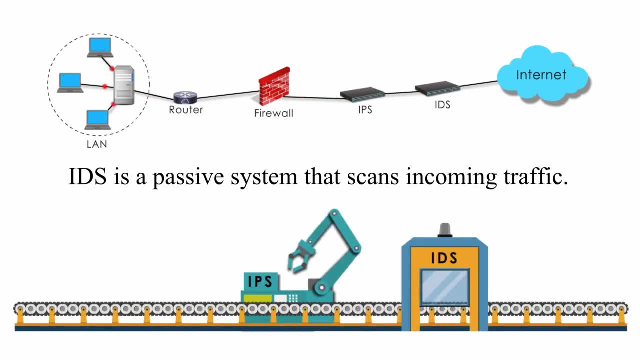 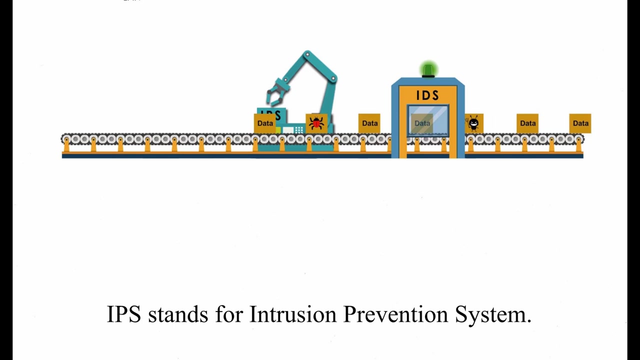 It can detect a CCTV camera above a business entrance or sensors on its doors. IDS is a passive system that scans incoming traffic. Once the IDS identified a dangerous or suspicious traffic, it can send alerts, but leaves the action to IPS. IPS stands for Intrusion Prevention System. 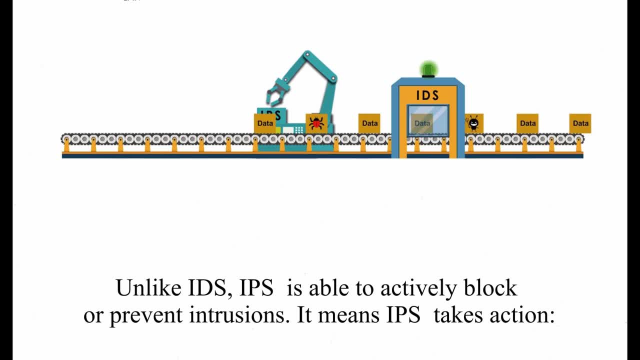 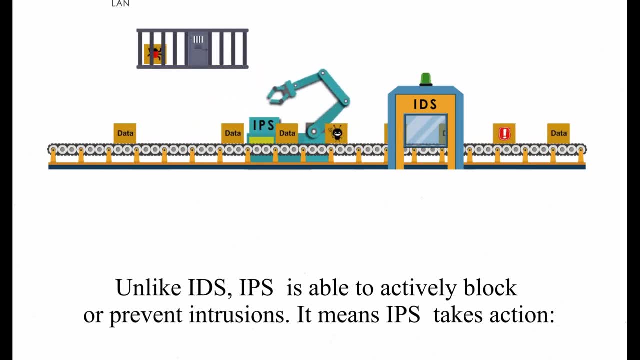 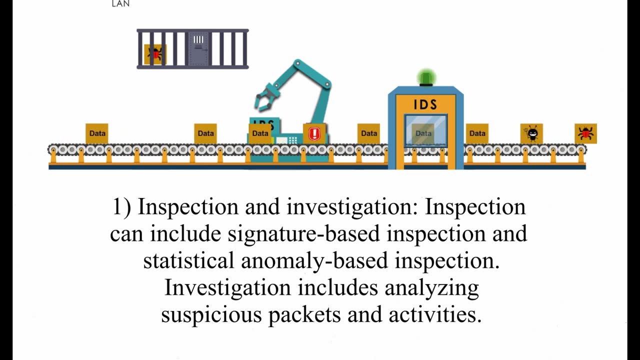 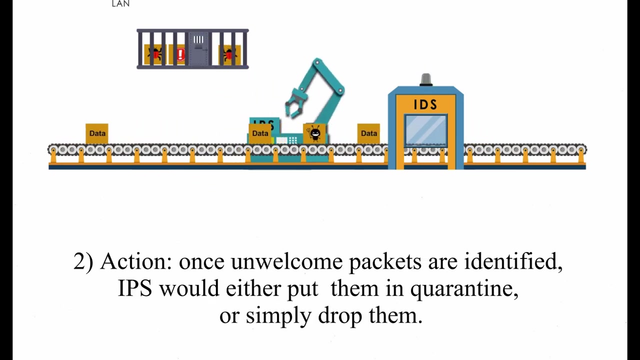 Unlike IDS, IPS is able to actively block or prevent intrusions. It means IPS takes action. One inspection and investigation. Inspection can include signature-based inspection and statistical anomaly-based inspection. Investigation includes analyzing suspicious packets and activities. Two action: Once unwelcomed packets are identified, IPS would either put them in quarantine or simply.